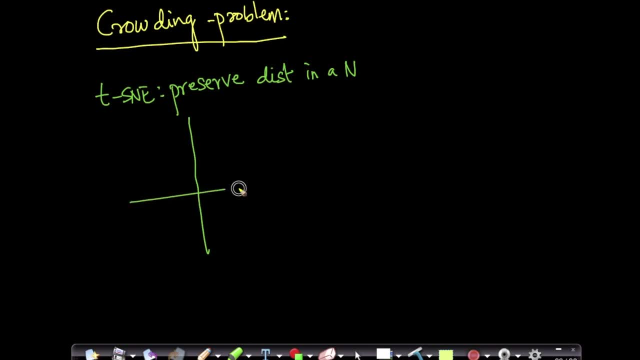 example, Let us assume I have two-dimensional data, okay, and let us assume I want to project this into 1D- okay, Let us assume I want to project this into 1D- okay, using t-SNE. okay, I want to embed these points. Suppose my four points, let us say, are: my first point is: 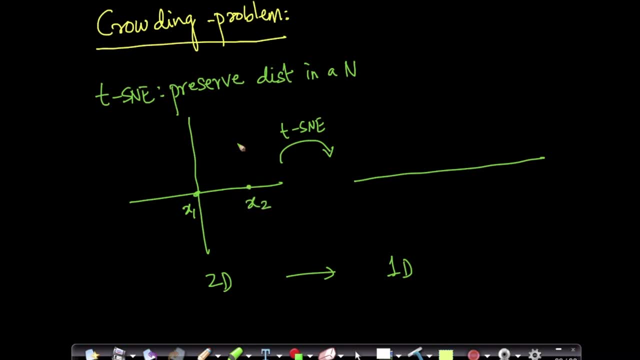 x1 here. my second point is x2, my third point is x3, my fourth point is x4.. Let us assume they are. they are corners of a square. okay. What does it mean? It means this length, this length is same. 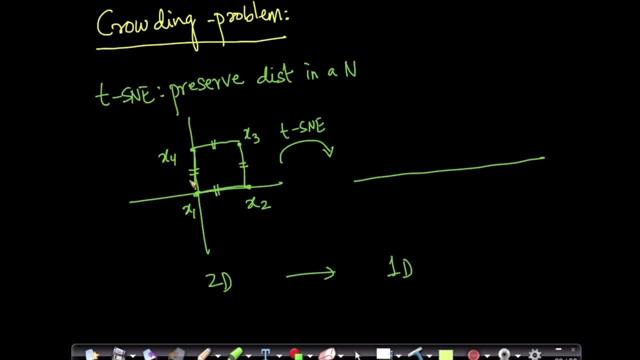 as this length, which is same, This length, which is same as this length. So if I have four points like this in 2D space which are equidistant, so all these points are equidistant right? So they are forming basically. 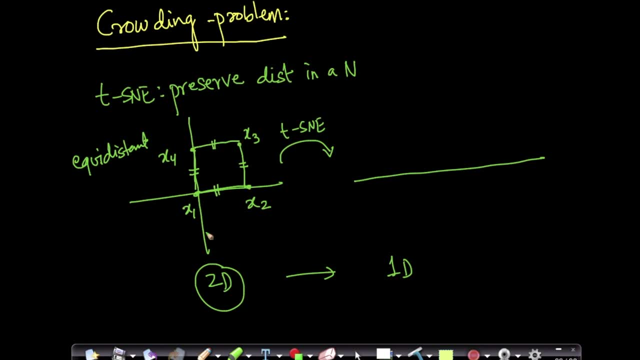 a square. okay, So this distance is same, as they are not equidistant from every other point. So let us, let us say: they fall on a square, right, If it is in 2D, it is a square In 3D. 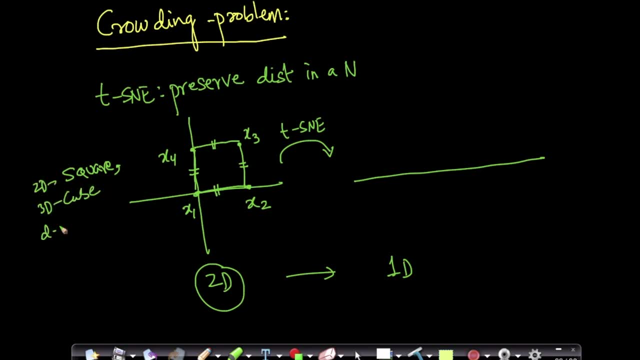 it is a cube In ND or in in d-dimensional space. it is a hypercube, right? We learned this in linear algebra, right? If I have points in in d-dimensional space, they will let us assume in 2D that they. 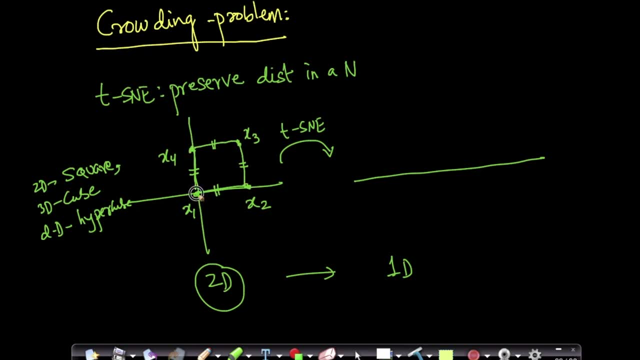 are. they are corners of. they are corners of a square. Now, if I want to embed them into one-dimensional space, let let us see. let us see the problem that we will quickly run into. okay, So let us assume I want to embed my x1,? okay, We will just do. this is a very simple. 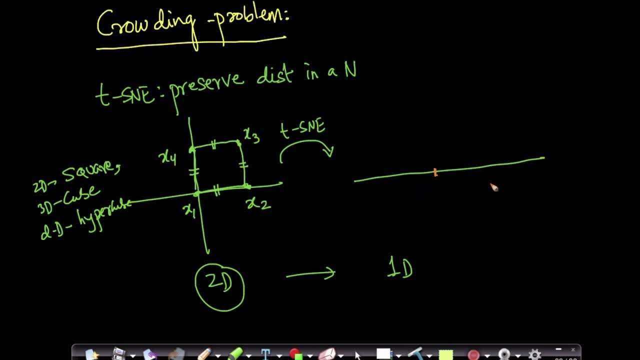 example, where I will prove that you cannot perfectly embed these points. okay, Let us see, let us go through that. So first let me put my x1.. I know that my x2, my x2 should be at at this distance. okay, at this distance. So I will place my x2 such that. 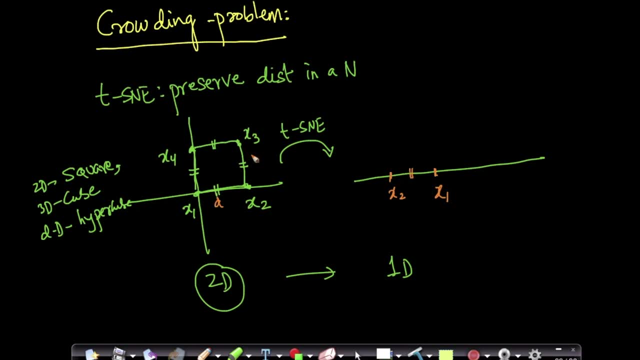 the distance between x1 and x2.. So, let us assume this distance is d. okay, Let us assume this distance is d okay, I will make sure that this distance is d. So I have embedded my x1, I have. 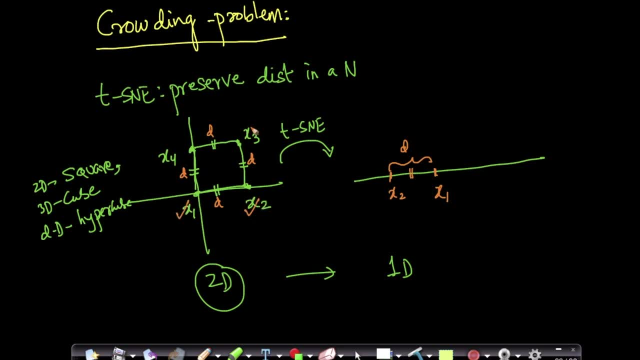 embedded my x2.. Let us take x3.. The good thing is x3,. x3 is at a distance of. x3 is a distance of d from x2, right, So let us say I, so I can embed. 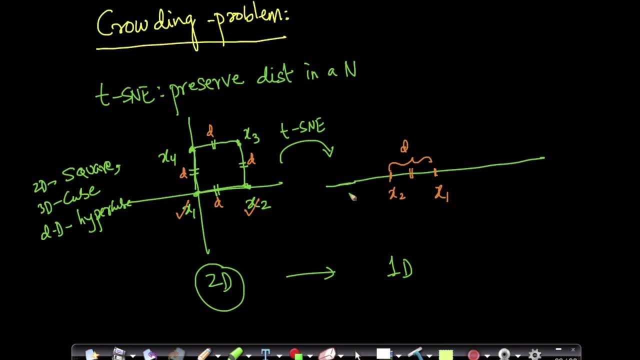 so I can embed my- sorry, I can embed my x3 here. Let us assume I am defining my neighborhood as points which are at a distance of d, which means x1 and x3 are not in neighborhood right, Only x4,. 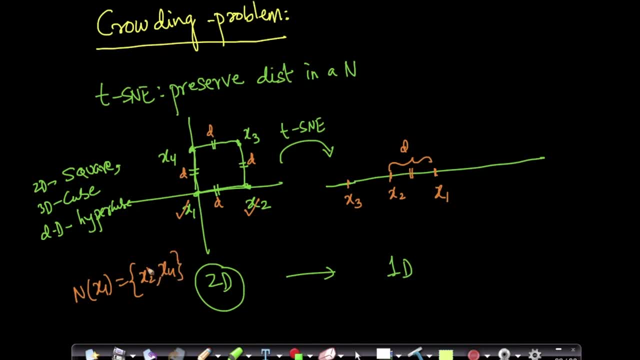 is x2 and x4, not x3, because this distance, this distance is not, is more than d right. This is square root of 2d right. This distance is square root of 2d right. So d square plus d square. 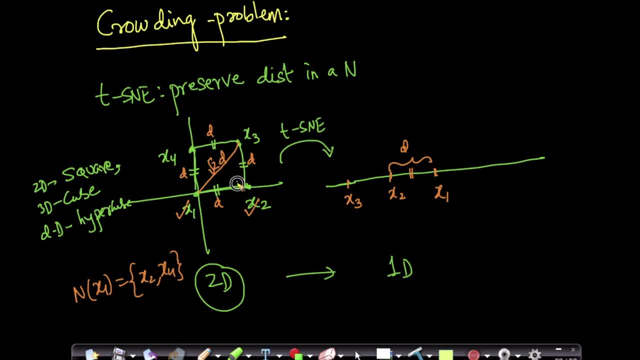 sorry, 2d square, yes, square root of 2d. yes, because this is a perpendicular line. This is: these two lines are perpendicular. Using Pythagoras theorem, this distance is root 2d, right? So let us say: 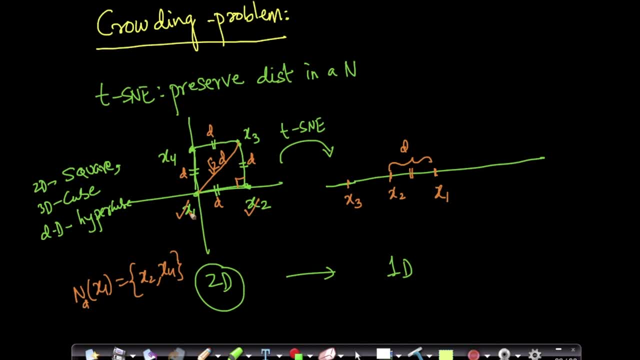 I am defining my neighborhood using distance d, Then of course I am preserving. I am preserving this distance. I need to just preserve these four ds. I do not have to preserve the distance between x1 and x3, because the distance between x1 and x3, okay, so this is also d. let us say. 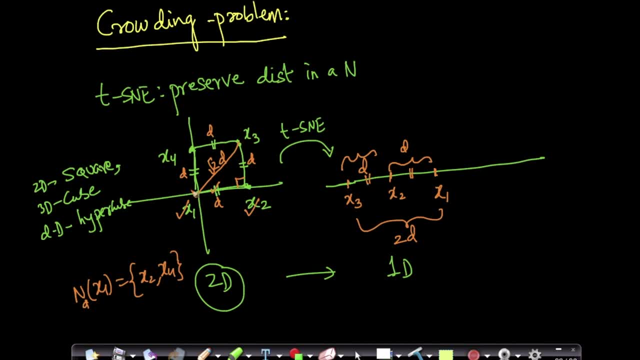 The distance between x1 and x3 is 2d, while in this, in the, in the, in the two-dimensional space, it is root 2d. But since, since x3 does not belong to neighborhood of x1,, 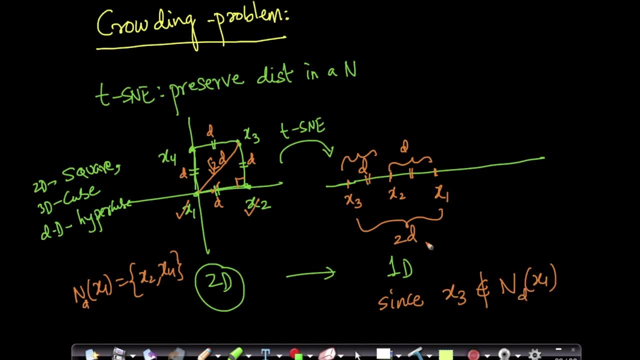 at distance d, I do not have to preserve it right. So this is perfectly okay. Placing x3 here is perfectly okay, But now comes the tricky part: What? where will I place my x4?? I need to place. 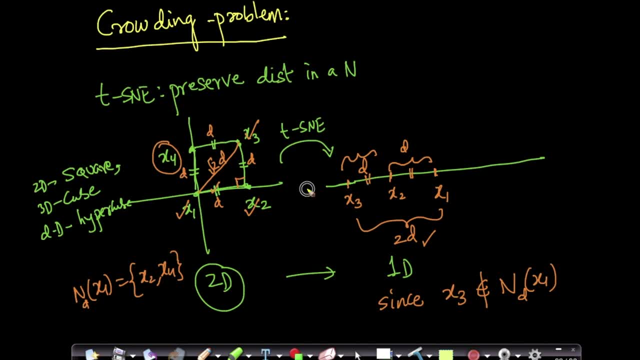 my x4.. So let us take multiple options here. okay. Let us say I place my x4 here, okay, at a distance of d from my x1, which means I am preserving this distance. okay, My x1, x4 distance. 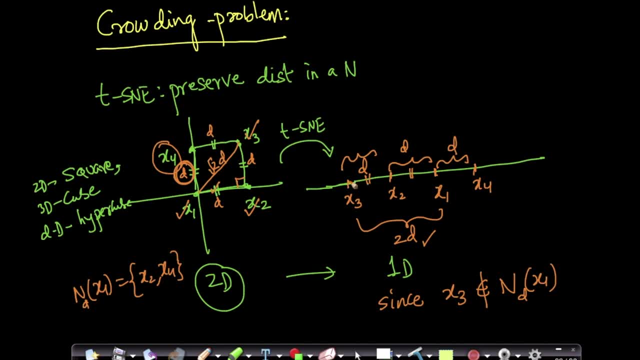 is what I am preserving. But as soon as I place my x4 here, my distance from x3 to x4 has become 3d, while it should be d. right, because my x4 and x3 are in a neighborhood, because my neighborhood of x3 is x4 and x2,. 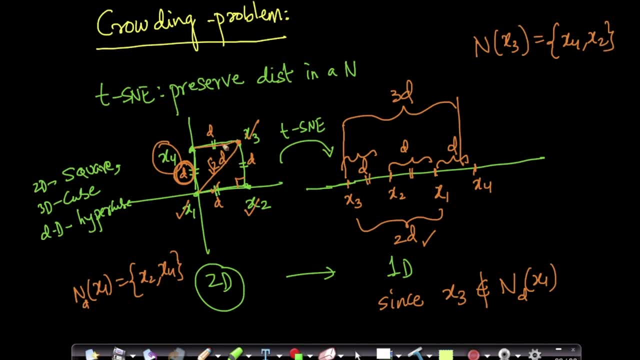 right for x3.. This is my x3. Its neighborhood contains x2 and x4, right, But where will I place my x4?? If I place it here, okay, my x1, x4 distance- x1, x4 distance is being preserved, but this is not being preserved. Similarly, if I place my x4, 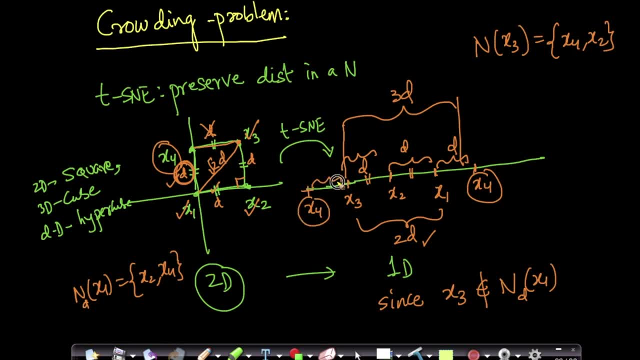 here. if I place my x4 here, this distance will be preserved, but this distance will become 3d now. So, whatever I do, if I have to place my x1, x2, x3, x4 points onto one-dimensional space, 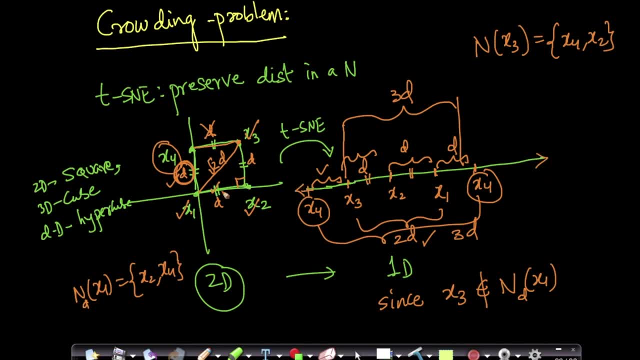 one-dimensional space is nothing but a line, right? One-dimensional space is nothing but a line. Whatever I do, okay, I will make at least one Mistake. right? We just saw it right that wherever I place my x4, whether I place here- 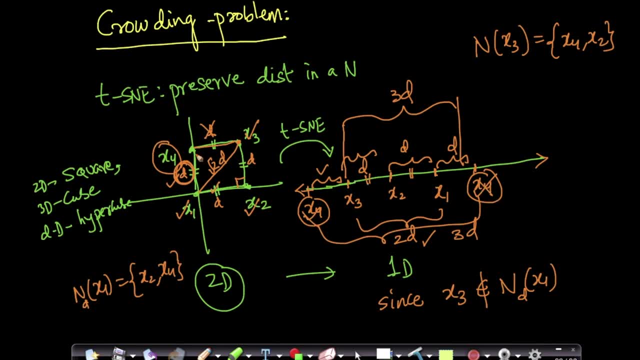 or I place here. neither of them will work because at least one distance- either this distance or this distance- will get corrupted. So there will be cases like this. So this is proof by contradiction. So I am taking a case where I have my data points like this and I am saying: 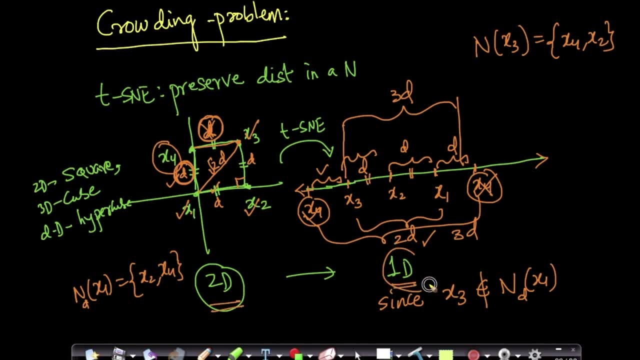 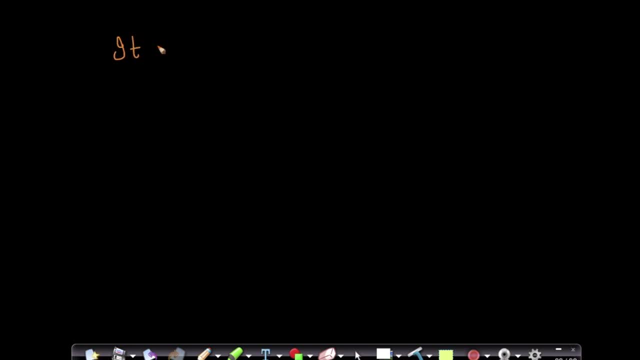 I will not be able to project this data from 2d to 1d by preserving all the distances in a neighborhood. So sometimes it is impossible, sometimes, sometimes- not always- sometimes, especially in the case of these hypercubes- it is impossible to preserve, to preserve distances in all the neighborhoods. 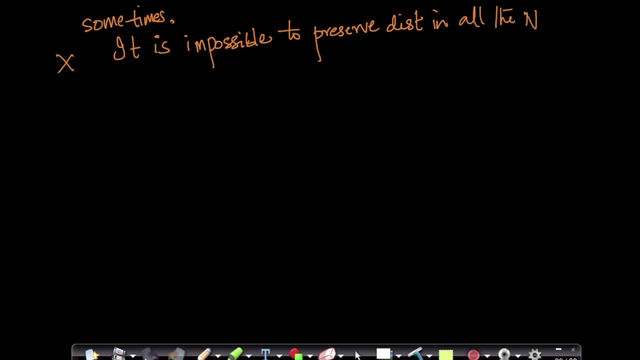 in all the neighborhoods. It is impossible, as we just saw. I proved it with contradiction right. I just took 2d data and I tried to project it into 1d and I just- and I just failed. Such a problem is called the crowding problem. 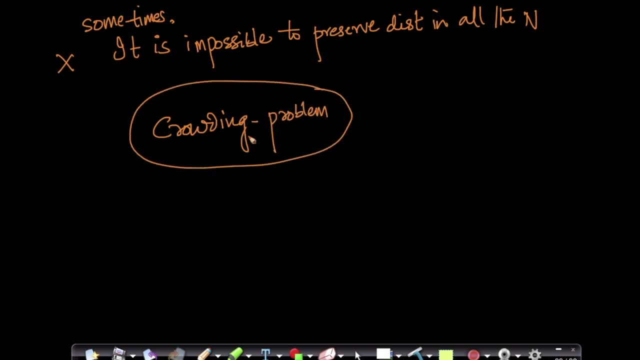 What it means is your points are getting crowded. that is impossible, Do whatever. So this is, this is this is one of the reasons. So earlier before t-SNE, I think a few years before t-SNE. 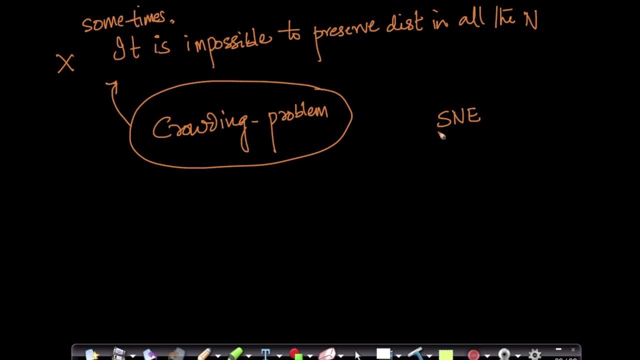 there was a lot of research on stochastic neighborhood embedding. Okay. Then people said when, whenever they did stochastic neighborhood embedding, they started observing this problem of crowding And then they said: let us use t distributed stochastic neighborhood embedding Again.